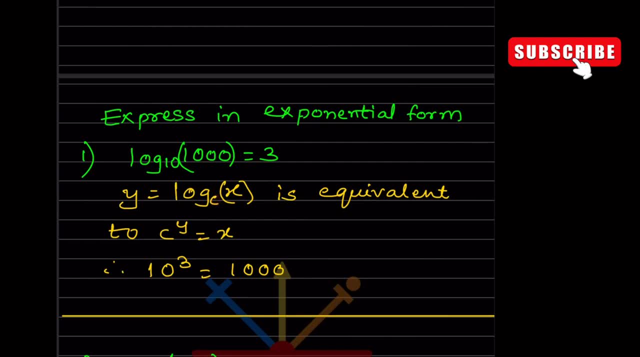 to log of x to the base. c is equivalent to c. rest to y is equal to x. so now I will write this one, so that is going to be c. c is here, that is 10. rest to y: this is y, so that is going to be. 3 is equal to x. what is x? x is 1000, so you can also see cross. 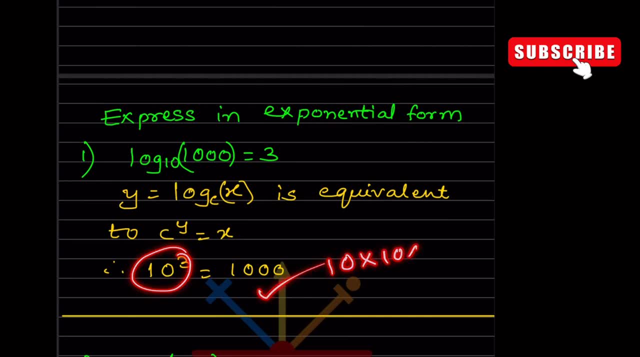 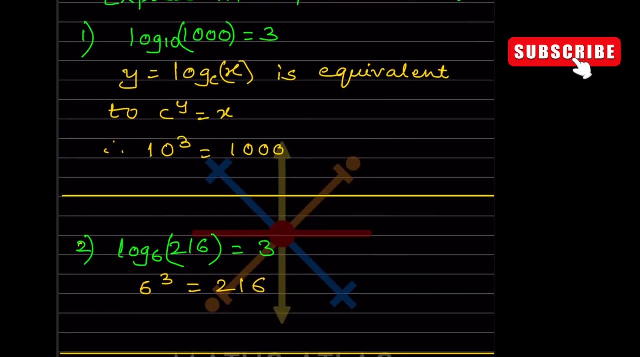 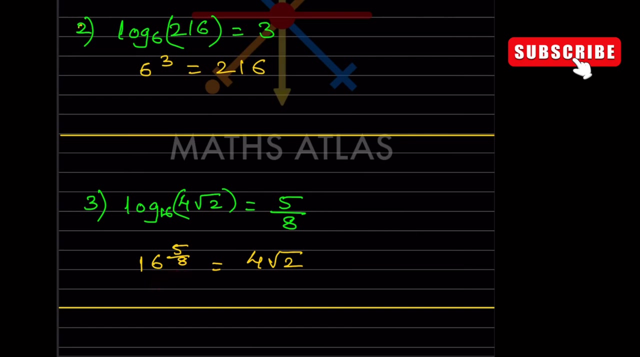 check: work 10 into you, multiply 3 times, you get 1000. so here again you are going to use the same formula. that is 6. rest to 3, that is 216. and this you can also cross check with this one, that is 216. so now here for this one. this is going to be 16. rest to 5 by 8. 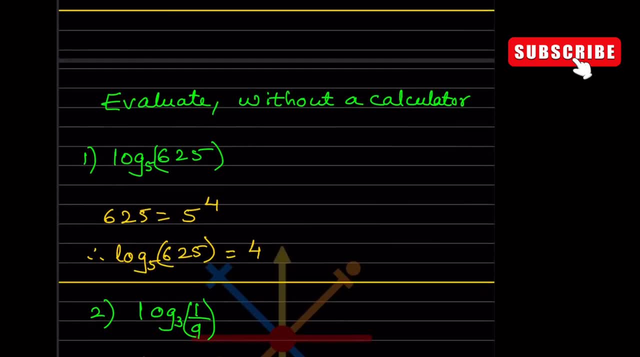 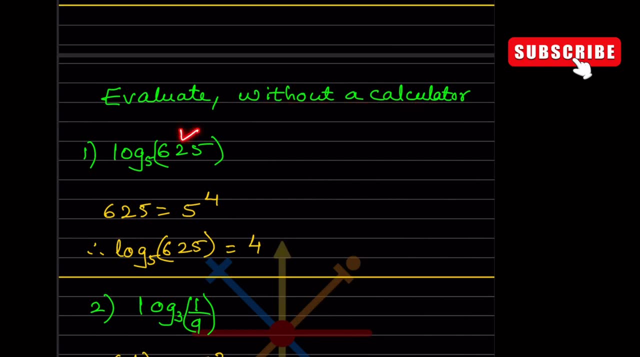 that is 402.. So now you have to evaluate. So now you have to evaluate. So now you have to evaluate this, but without a calculator. so this is important here. so how are you going to write here? so 625 is equal to 5, rest to 4. so you are going to write. 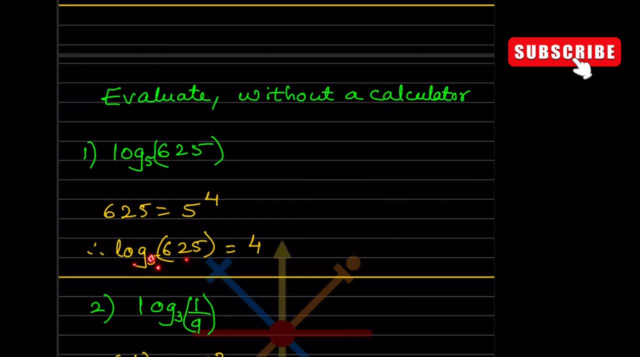 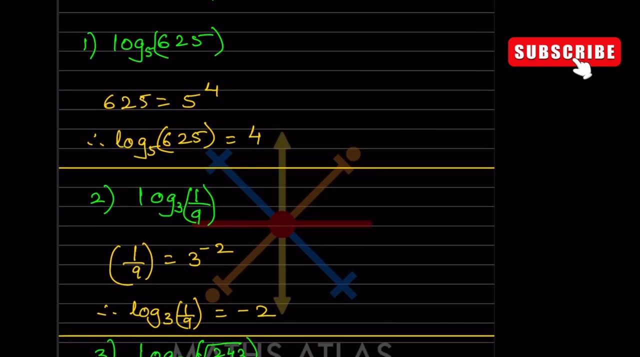 here: log of 625. rest to the base 5. that is, 4. same over here. how will you write this one log of 1 by 9 to the base 3? that is going to be: 1 by 9 is equal to 3, rest to minus 2. 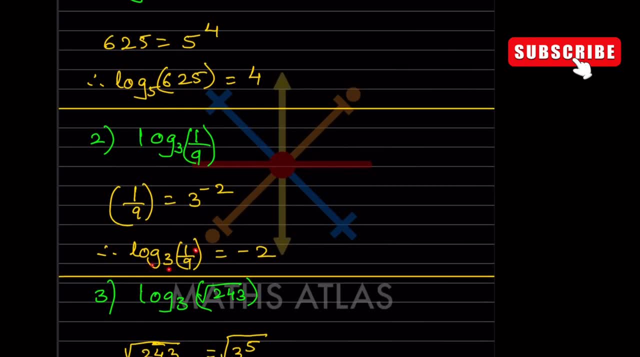 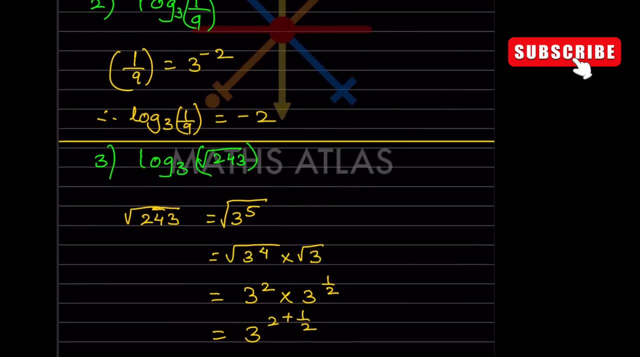 so here you can write here log of 1 by 9 to the base 3, that is minus 2.. Now look at here log of root of 243 to the base 3.. So log of 243 that is going to be. you will factorize that 1.. 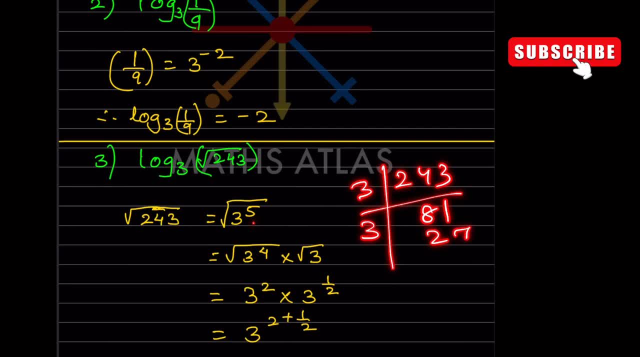 When you factorize this you are going to get 3 rest to 5.. So this three rest to five can be also written as 3 rest to 4 into 1 by 9.. That is 3 rest to 2.. root of 3 raised to 4 into root of 3 raised to 1. root of 3. because here, whenever we write, 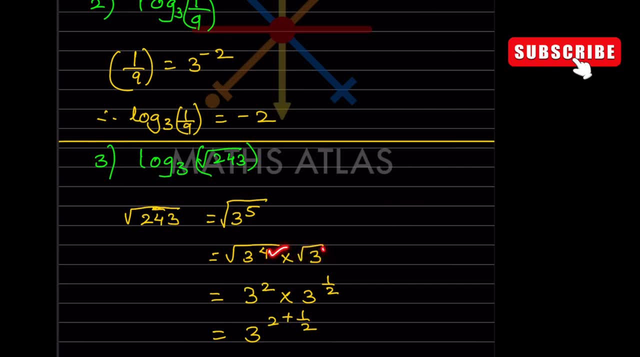 root of 3 means the exponent is 1. so 1 plus 4, that is going to be 5. so now see here this: when you take the root of this one, so that is going to be 3 square, and this is when you remove the root, that is going to be 3 raised to 1 by 2. so now this, because you know the. 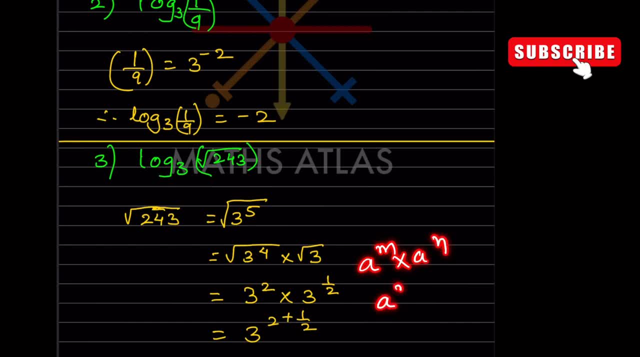 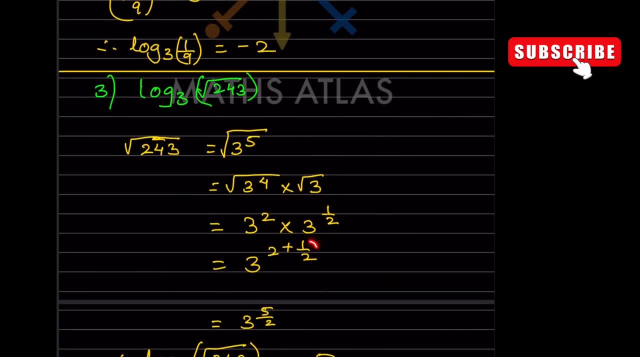 exponent rule, a raised to m into a raised to n, that is, a raised to m plus n. so here you are going to add the exponents because the base is the same. so this is going to be 2 plus 1 by 2. so you take the LCM of this one, so that will be 4 plus 1 by 2, so that 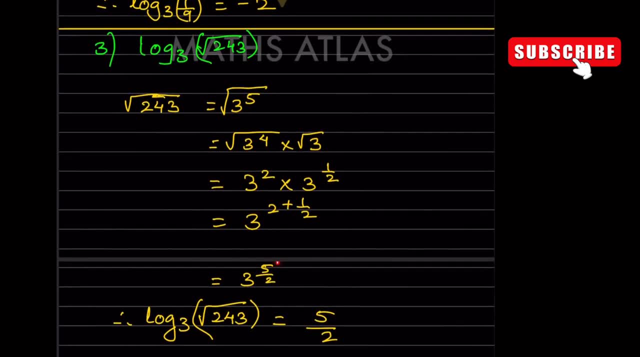 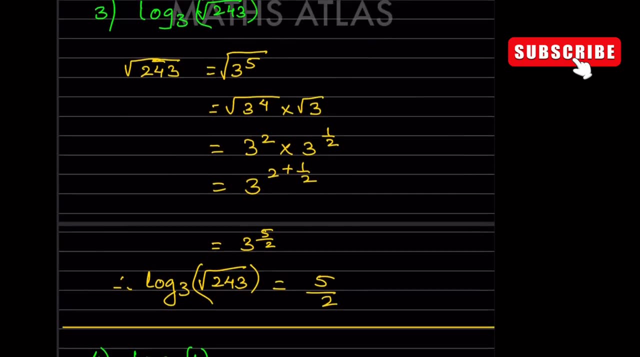 is going to be 5 by 2, so that will be 3 raised to 5 by 2. this is only for root of 243. we got as 3 raised to 5 by 2, so now how are you going to write this one? 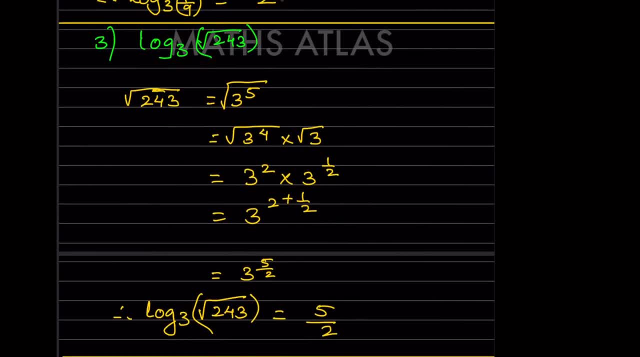 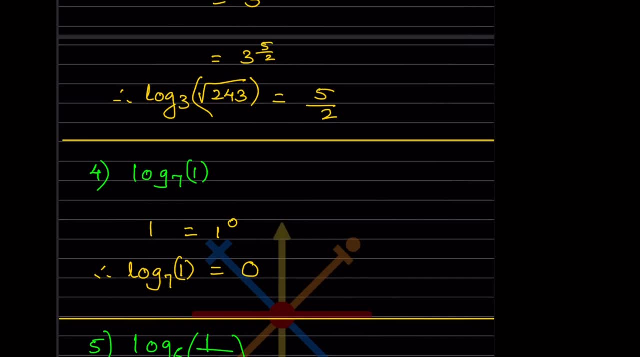 So will write here, therefore, log of root of 243 to the base 3. that will be 5 by 2. so now this is a bit different log of 1 to the base 7. so this one, we can also write this one as 1 less to 0, because anything less to 0 is 1. even if it is 99 less to 0, that is going to be 1. 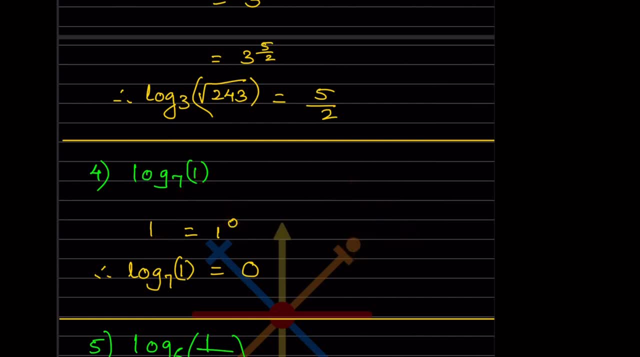 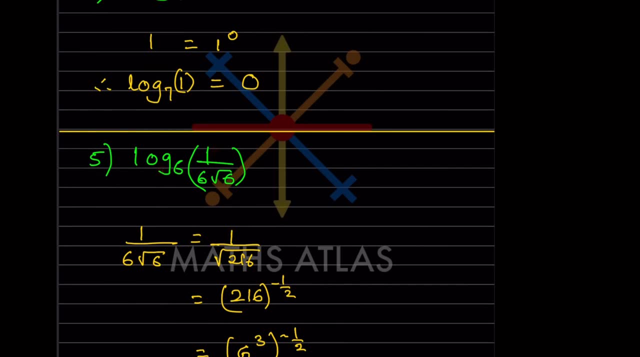 so now we can this right here, so we can write here log of 1 to the base 7. that is going to be, that is here 0. so log of 1 by 6 root 6, that to the base 6. so first thing, let us take this one. 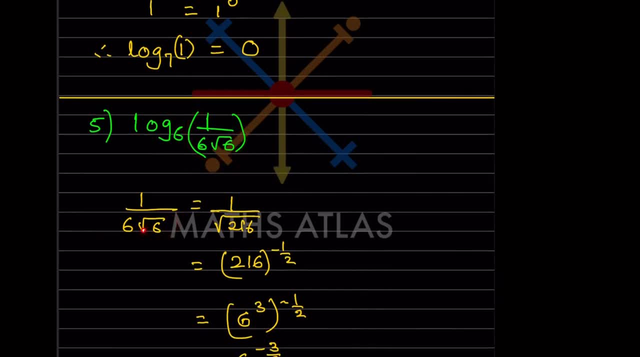 1 by 6 root 6. so when we take this we write the 6 root 6. root 6 is already there. when you take this in the root, that is going to be 6. is that 36? so now 36 into 6. that is going to be. 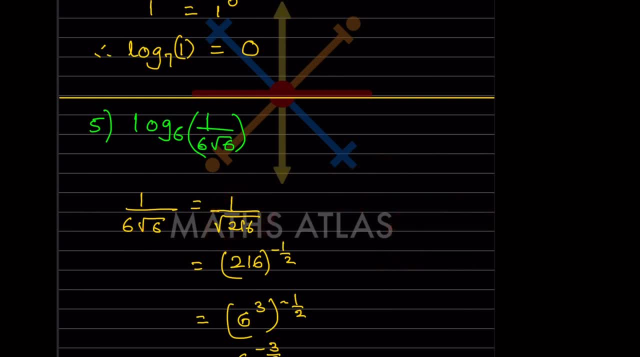 216. so this is 1 by 216 root of. so now we were going to remove, we can also write one step for this one. we can also write here 1 by 1 into: we are going to remove the root here. so what, we are going to write here one step you can write here. sorry for this. 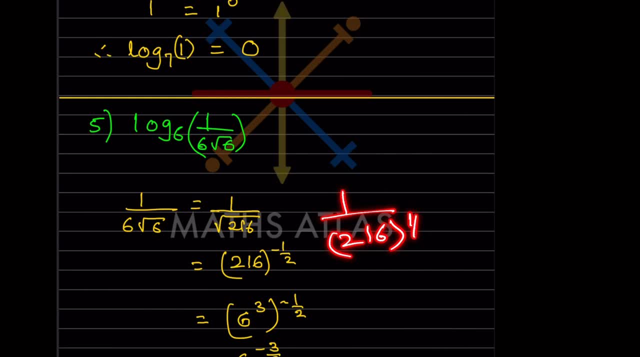 one. so we can write here: 216. rest to 1 by 2. and then when you flip over this one, when you take this in the numerator, so that is going to be 216. rest to 1 is 1 by 2. hope this is clear. so now, 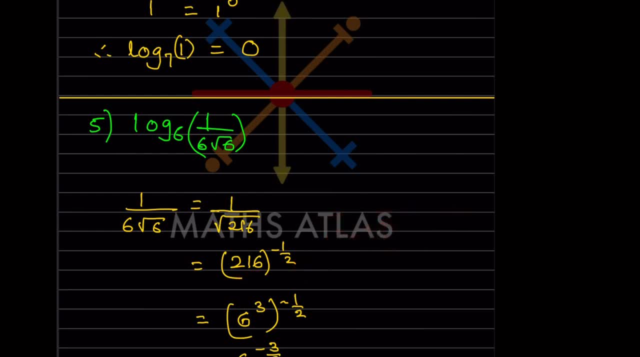 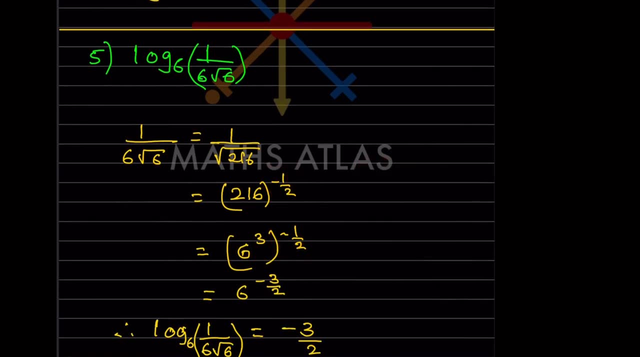 for 216 we can take. when you factorize it, we get 6 into 6 into 6, so that will be 6, rest to 3 and this will be minus 1 by 2. so what we'll do when you multiply this, a rest to m into n. 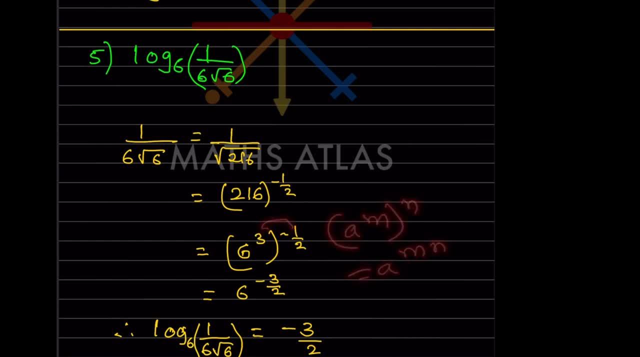 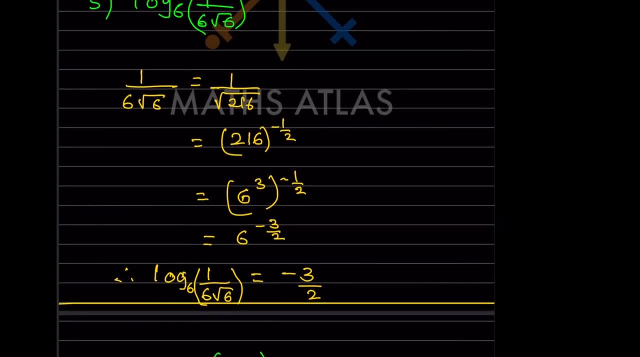 that is the a rest chairman in exponents now. so that will be 6 rest to here minus 3 by 2. so therefore we can write the log of 1 by 6 root 6 to the base 6. that is minus 3 by 2. 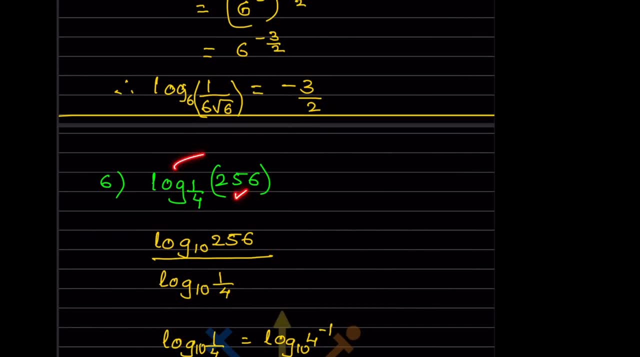 now this: we can also write this one as log of 256. always there is nothing is there means that will be. base is going to be 10 and this one log of 1 by 4 to the base 10. so now what we can do here. 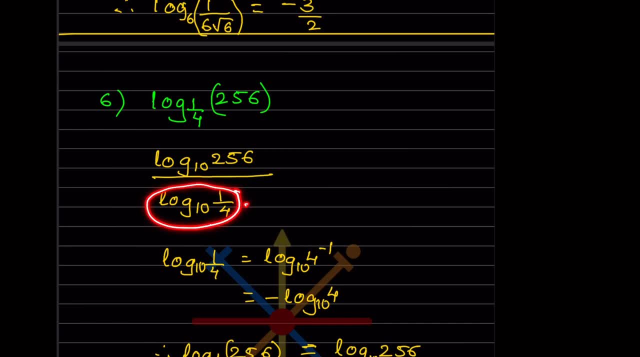 let us simplify this one, so this will be log of 1 by 4 to the base 10, so we can also write this as 1 by 4. we can write as 4 rest to minus 1. 1 by 4 is 4 rest to minus 1. 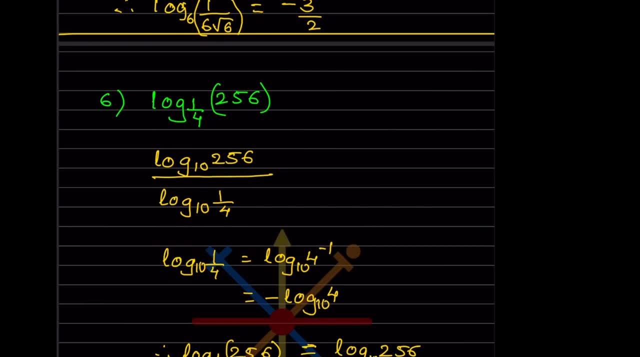 this is log of 10. as it is log of 4 rest to minus 1 to the base 10. so now what we can do here, we can write this one as this we can take as minus 1. this is minus 1 over here, so actually. 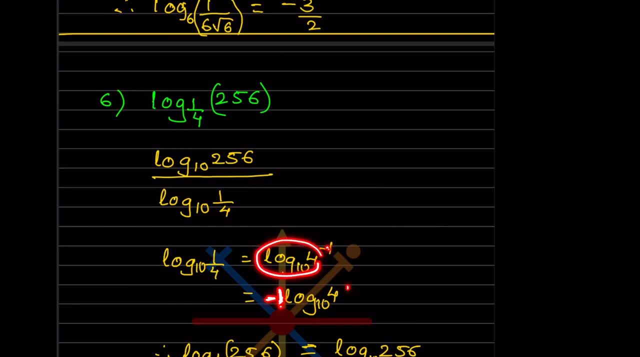 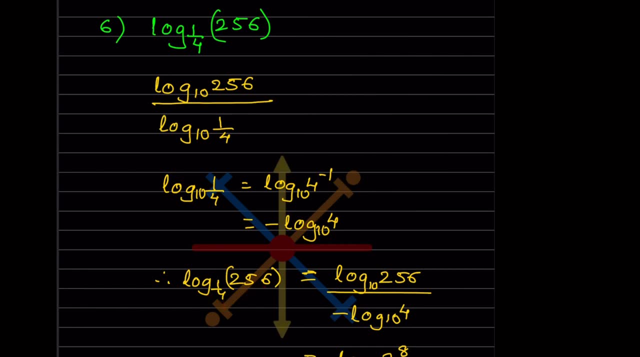 we don't write 1, so that is just minus over here and this will be the same. so now we can also write here: log of 256 to the base of 1 by 4 is 2, 1 by 4. this is pressing this off. this is like it is and for this one, what we have done, we have. 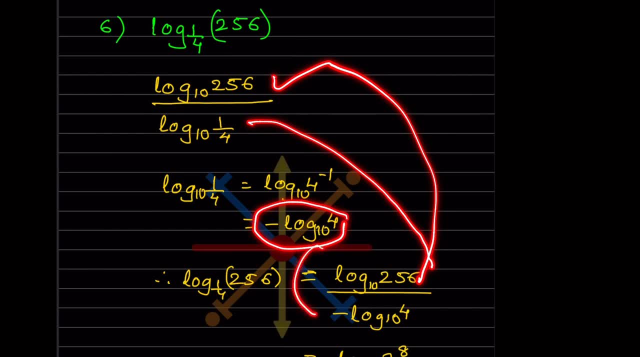 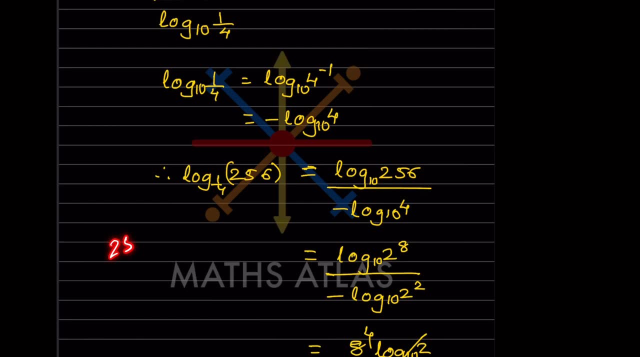 simplified this one and minus log of 4 to the base 10. so this is what is here. so now, what will you do here? this, now 256. when you factorize this 256, you get t-raised to 8. you can factorize and see when you keep on. 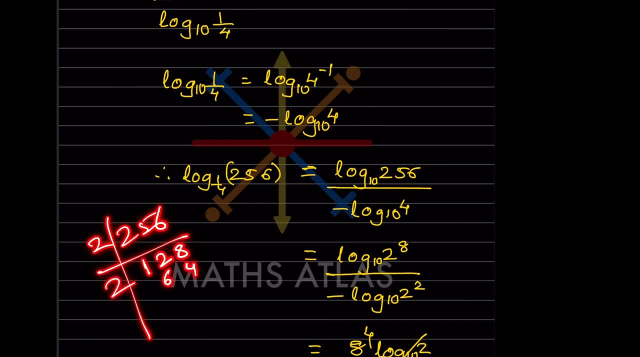 multiplying to, ones are to, twos are two, eights are two, 6s are twos say two. thirty twos are two, 2, 16s are 2, 8s are 2, 4s are 2, 2s are and 2, 1s are. so 1, 2, 3, 4, 5, 6, 7, 8, that will be 2. 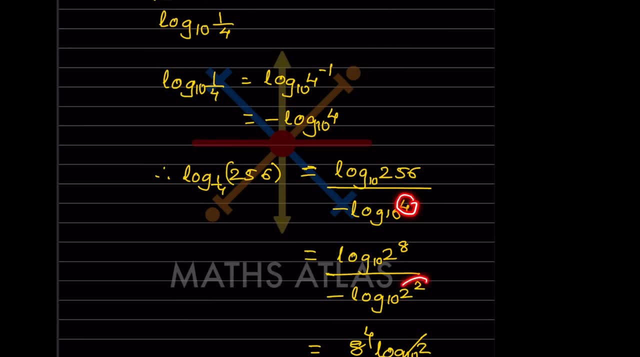 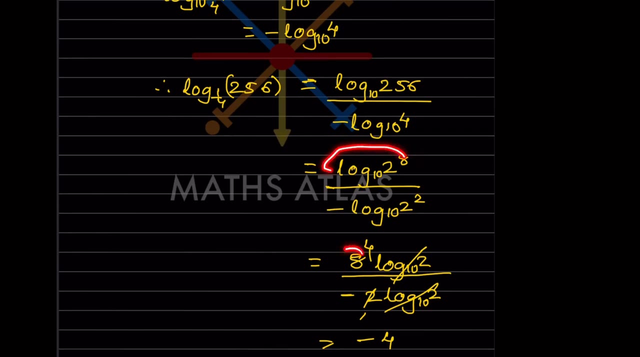 rest to 8 and this 4 can be written as 2. rest to 2. so now this minus is over here. rest: this is the same. so now here what we can do here. this is the exponent over here. so you know the rule. this exponent can be brought over here and this will be same here, the exponent. 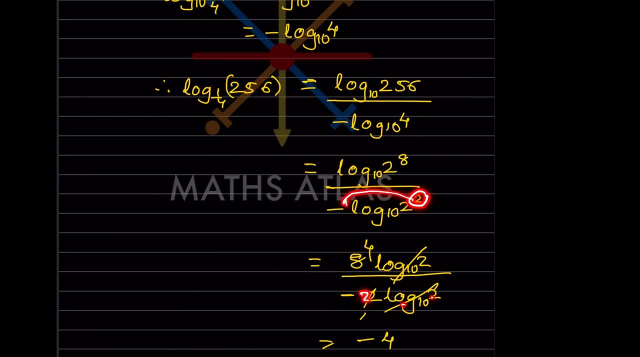 is 2, so it can be brought over here. that will be 2 log of 2 to the base 10. so now what you can see, this also is log of 2 to the base 10. this also is log of 2 to the base 10. so 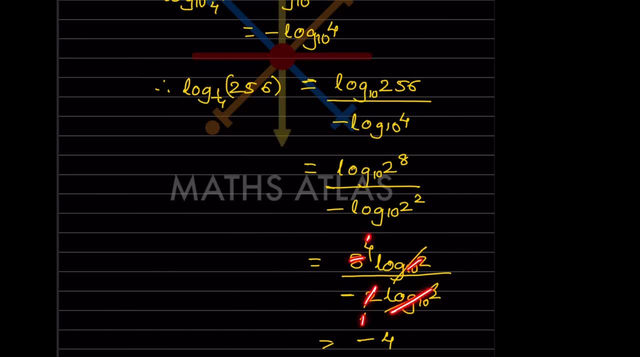 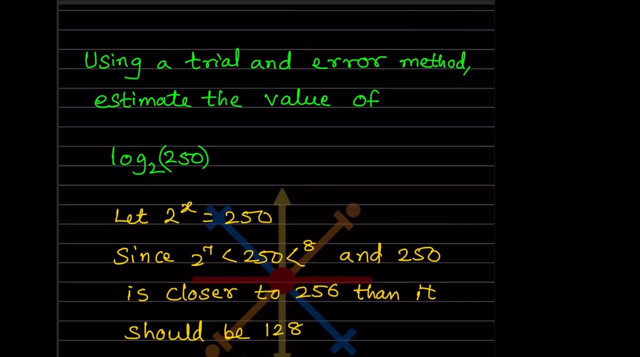 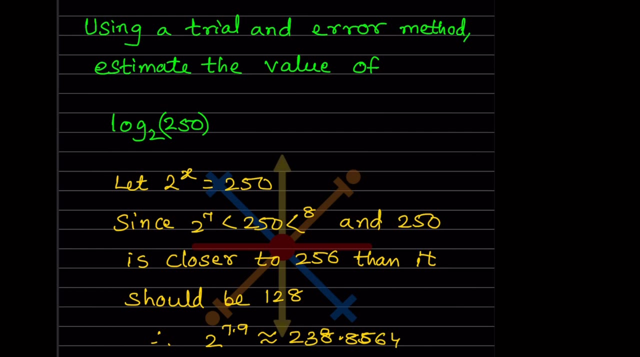 now we can cut off this one and then 2, 1s are 2, 4s are. so here is actually minus, so minus here. so answer will be minus 4. now, using a file and error method, we are going to see the method estimate the value of log of 250 to the base 2, so we can write that we can. 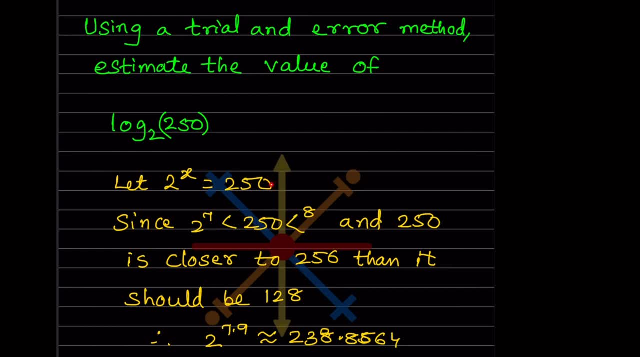 consider: let 2 rest to x is 250. so now here 250. you know this can be 2 rest to 8, that is 256 and that will be so. this 250 is going to align between 2 rest to 7 and 2 rest to. 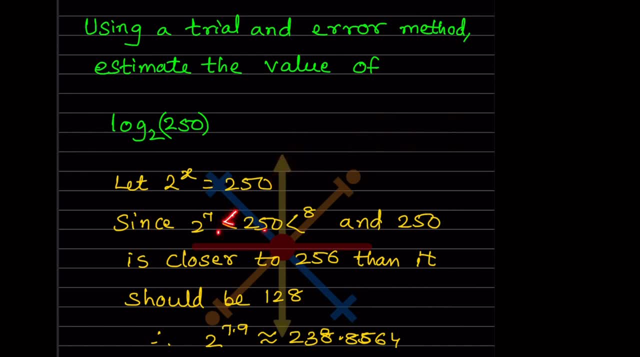 8. so since 2 rest to 7 is less than 250 is less than we can write, that 2 rest to 7 is right here to this to 8, and 250 slows. actually, this is 250. this 250 is closer to 2. this to 8 is what that is, 256. so we can consider this to this to 8. so now, 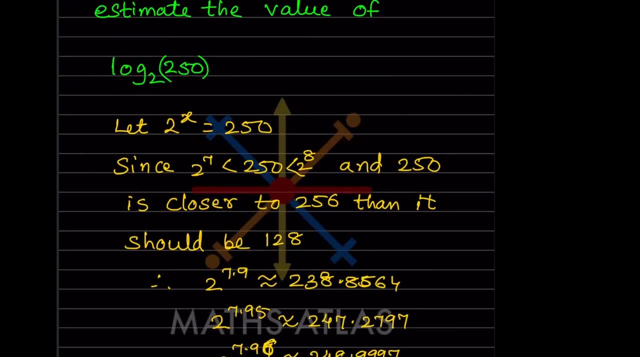 here to this to 8. so now, closer to that means it is going to be somewhere we can take care to this- to 7.9, that will be approximately equal to this 238. point 8: five, six, four, if we take care to this, to seven, point nine, four, that will be. 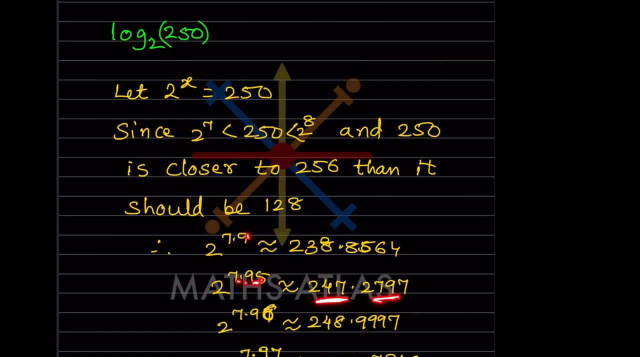 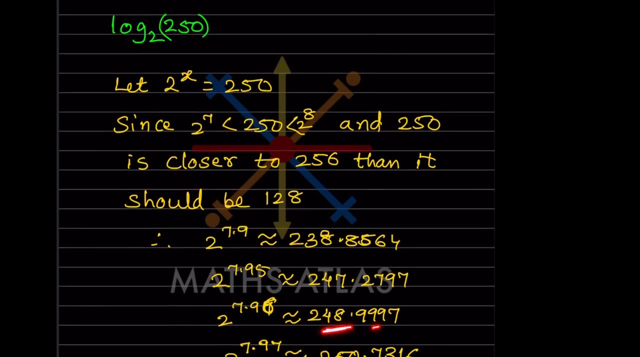 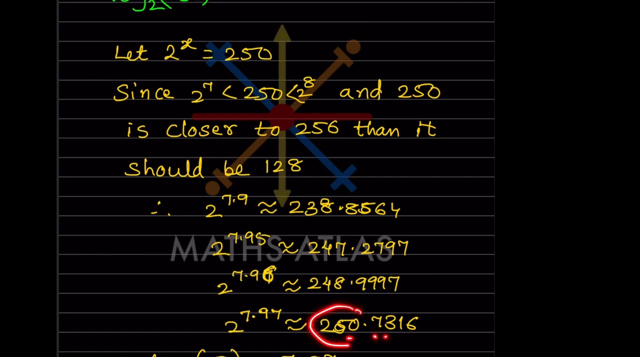 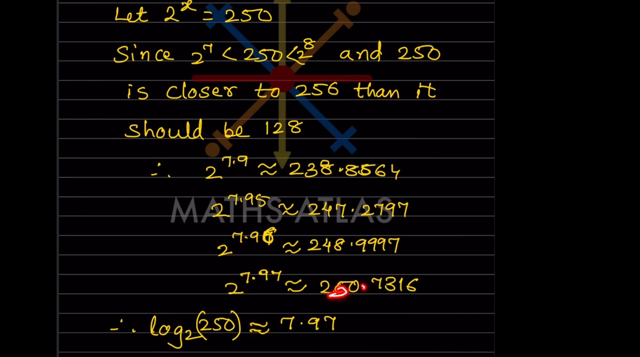 approximately 246 point. here again, if we take your 7.96, that will be 248 point here. if we take seven point nine, seven, so that is going to be 250 pointم. that is crossing 250. so now what can I do? to consider this will be approximately equal to, but here it is slightly more than 250.73. 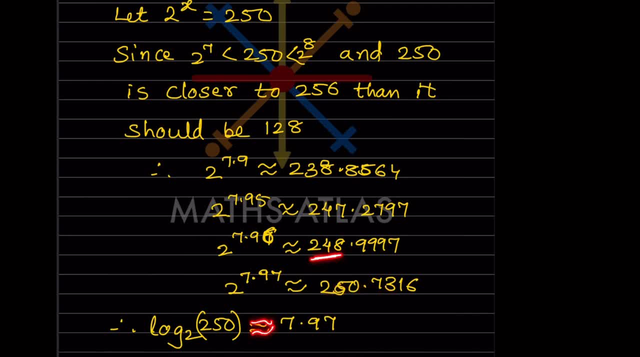 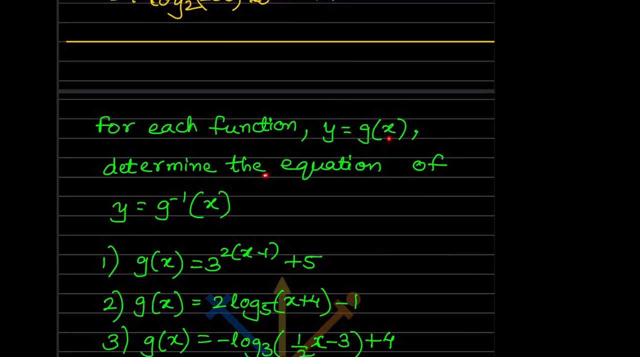 so that will be approximately equal to, because this is less 248, so this is just slightly more. so we can consider log of 250 to the base 2. that will be approximately equal to 7.97. for each function, y is equal to g of x and you have to determine the equation of. 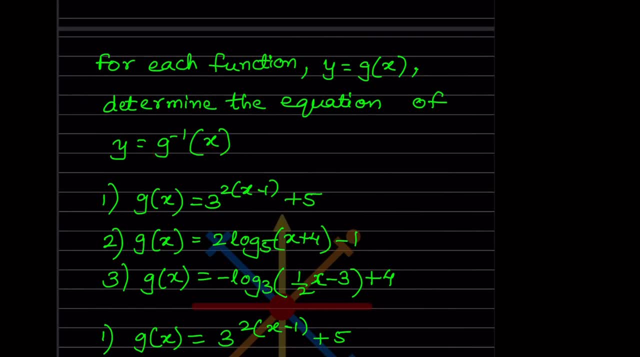 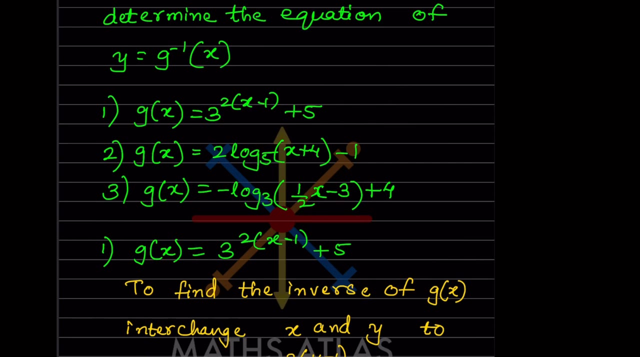 y is equal to g, inverse of x. so now, here we are going to consider this. 3 examples, that is, g of x is 3 raise to 2 x minus 1 plus 5. this and this equation. now let us first see the first part. so that is 3 raise to g. raise to x is 3 raise to 2 x minus 1 plus 5. so now 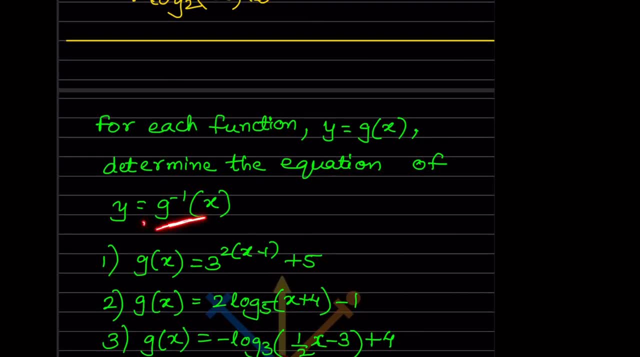 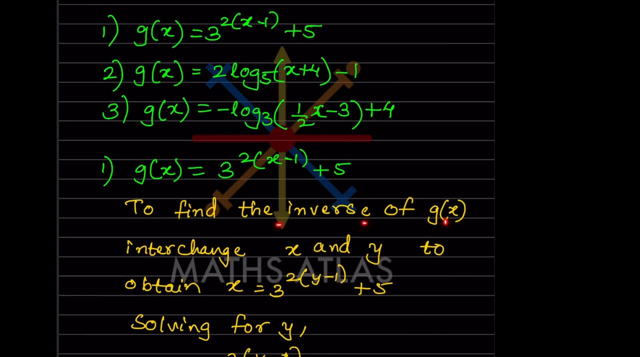 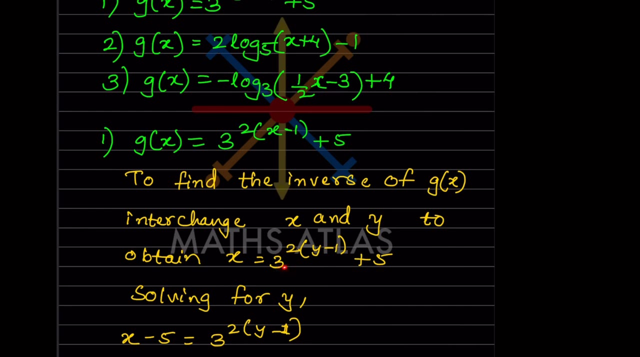 what are we going to do? we have to determine the value of this inverse that is y, is g inverse that is x. So now you have to find the inverse of g of x. what we have to do, we have to interchange x and y to obtain x is equal to. that is 3, raise to 2 y. so this is actually what this. 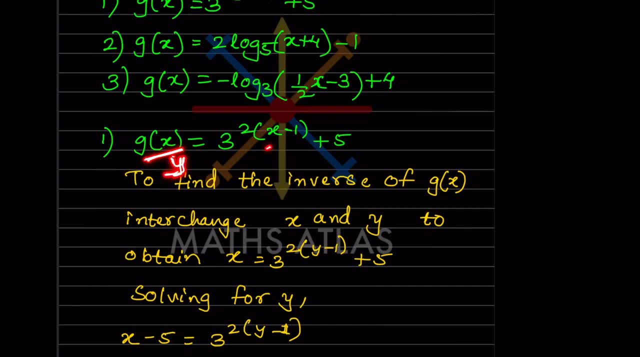 is y. so wherever you see x there, you are going to put y, and wherever you see here again, you are going to put here y. so now, what will you do here? this we are going to this is y, actually y, so you are going to consider this as x and this is x. so you are going to consider this. 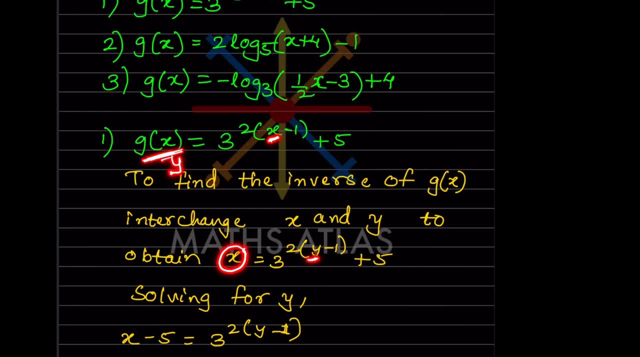 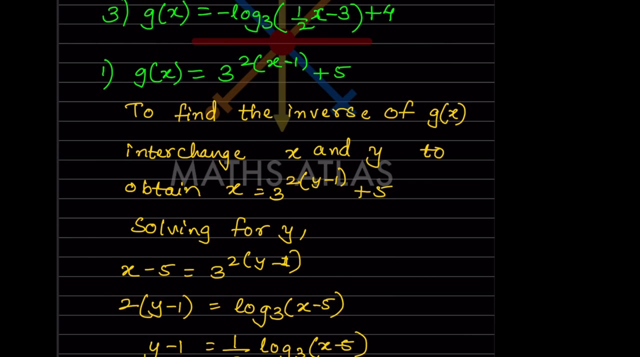 as y. Rest, all is the same. hope you got this. you have to interchange between x and y. so this way, if, even if it is g of x, that is actually y, so we are, you caught at x and this you got as y, so now we are going to solve for y. so now, what will you do? this plus 5 we will bring. 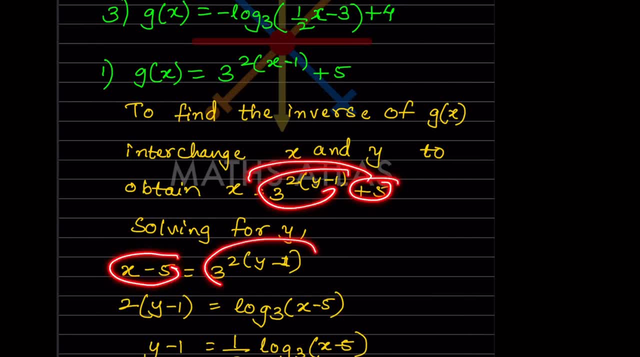 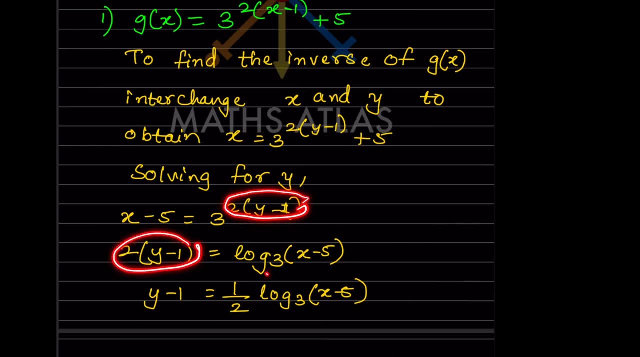 it on this side. so that will be x minus 5, and this is going to remain the same. so now, what will you do here? this is the exponent, so this will be here. according to the law, that is log of 5.. Log of 3 to the. this will be into x minus 5. so what will you do now? you will take your. 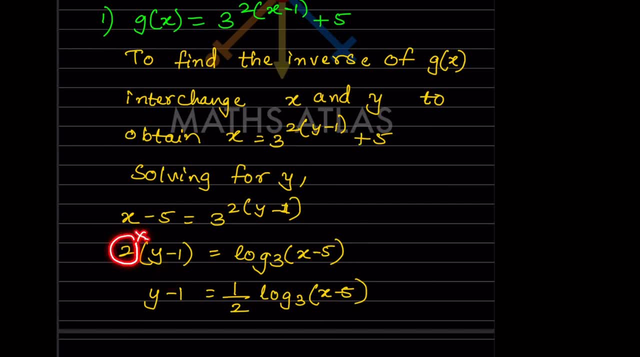 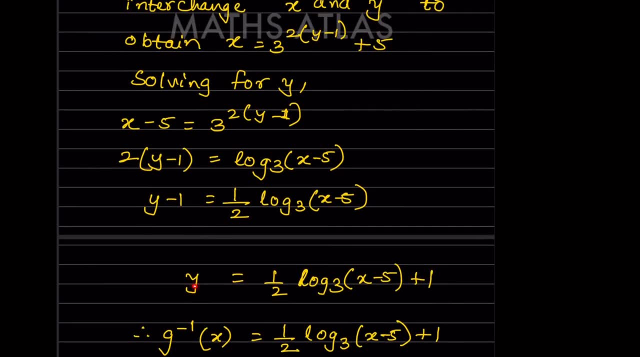 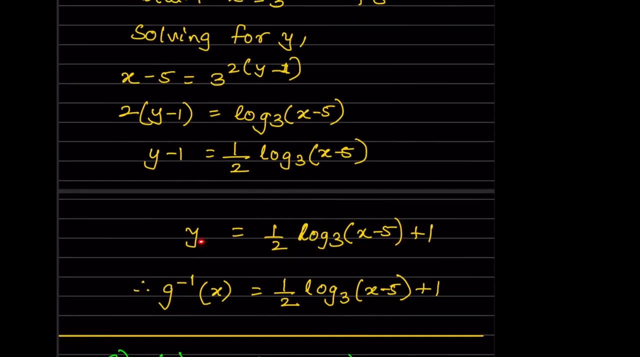 y minus y on this side and this 2 will go, because this is multiplication the other side. that will be 1 by 2, log of x minus 5 to the base 3. so now let us take here y, so this minus will go here, rest all will be the same. so y is nothing, but x is g of x, but y is not. 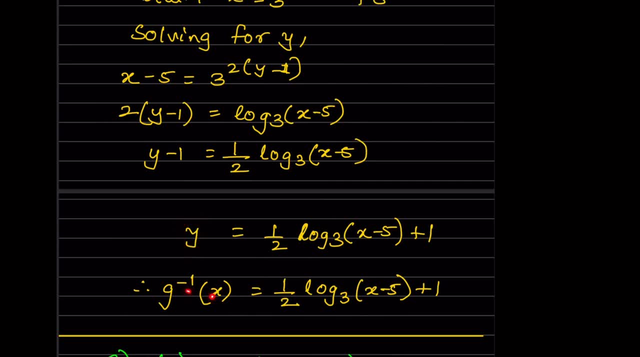 this will be g, The inverse of x. so now, what will you write here? this will be 1 by 2, log of x minus 5 to the base, 3 plus 1. so this is the answer. now the next one g of x is 2, log of x plus. 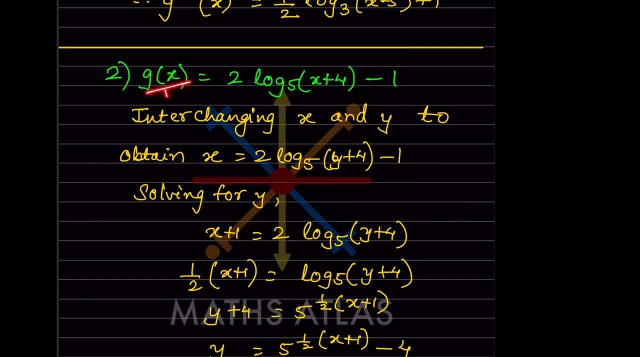 4 to the base 5 minus 1. so now again, this is y. so what are we going to? we are going to interchange in x and y to obtain: x is equal to this. y means this will be x and this is x means this is going to be y. rest, all is the same. 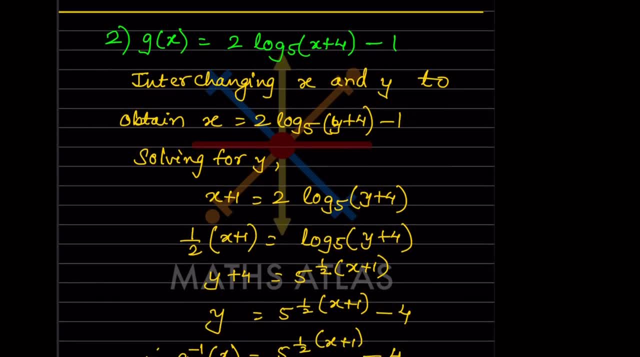 This is what is written here. then you are going to solve for y. so what will you do? minus 1, you will take on this side. so that is going to be plus 1. rest is the same. so now this 2, if we take it on this side, that is going to be 1 by 2 and this will be the same. the 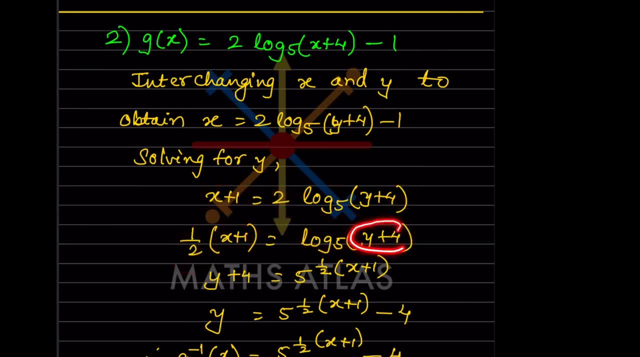 same. so now what you can do here. this y plus 4, you are going to bring it here, so that will be what y plus 4 is: 5 and this 1 by 2 will go in the exponent and this 1 by 2 will go. 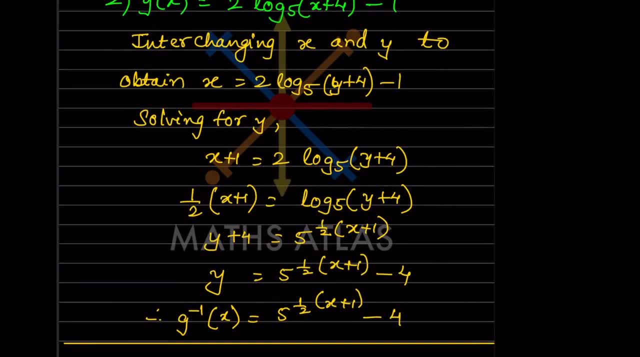 in the exponent. This is x plus 1. so now you want the value of this y, so plus 4 will go. on this side, that is going to be minus 4. so this remains the same. so y is what that is. g inverse x is this: 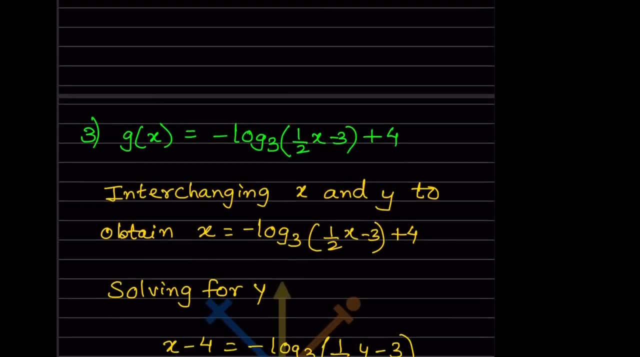 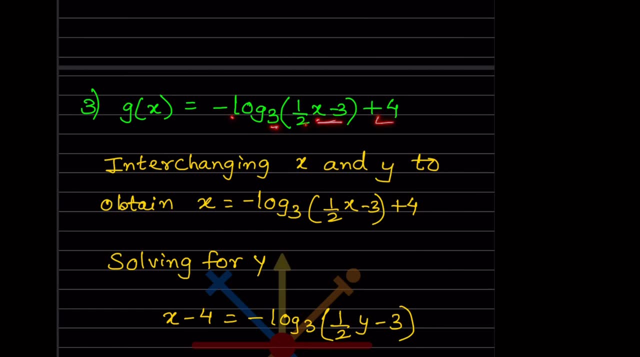 whole part. so now the next one, g of x is minus log 1 by 2 x minus 3 to the base 3 plus 4. so you are going to interchange x and y to obtain. so now, what are we going to do? again, this y is going to be x and this x is going to be here. you are going to write here: y, sorry. 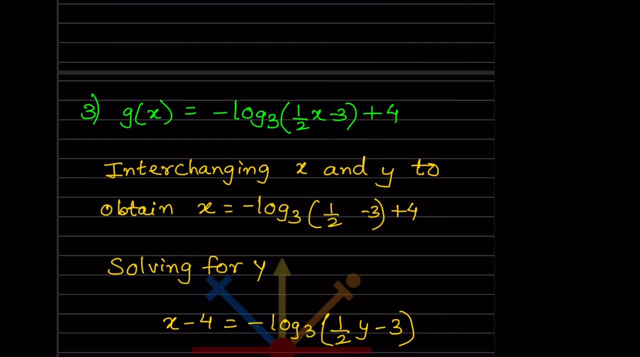 for this. so this is y. so now you are going to rest. all things are going to be the same. so now you are going to solve for y. so now plus y will be here. so that is going to be minus y, and this remains the same. 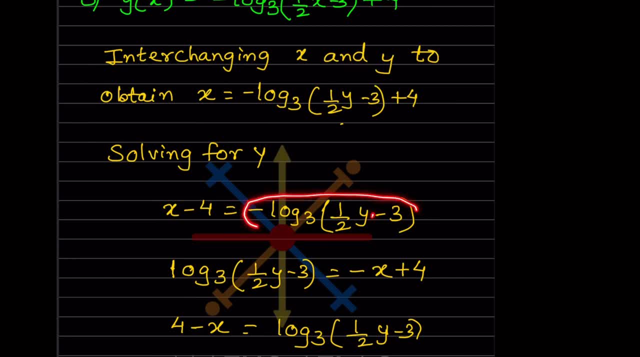 so now, what will you do? this thing, this minus, will this whole part, because this is minus, it will go on the other side, so that is going to be plus. and what will happen here? this is: this is plus x, so this is going to be minus x minus 4, so this is going to be plus 4. 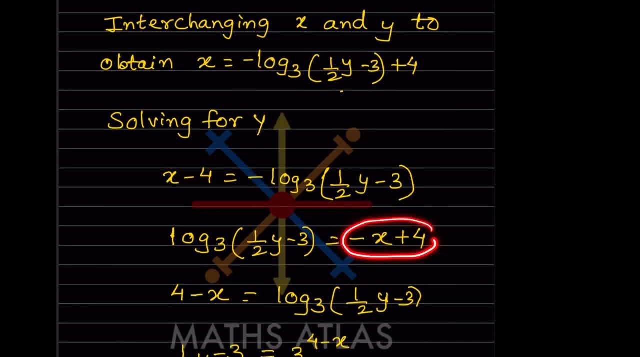 so what we can do here, we can also write this, as we will take this on this side both the same, and this will be this side, so we are not going to change any, the sign only. we are going to change the total, we are going to change the place, so that is not going to change the sign. 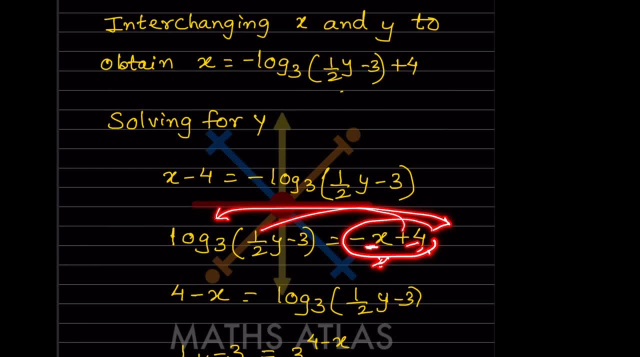 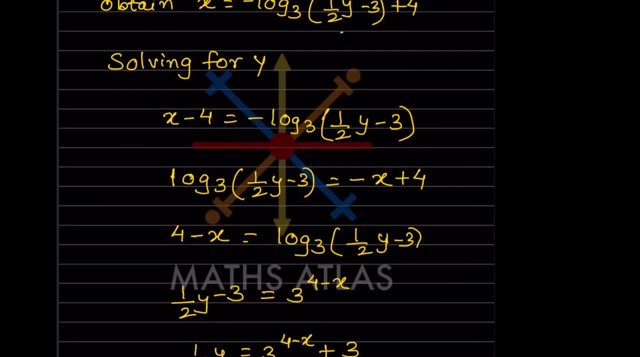 so now we can write here, because we want here 4 in the start and minus x over here. so now this whole thing is here. so now here what we can do. here we can write a 1 by 2, y minus 3 is 3. 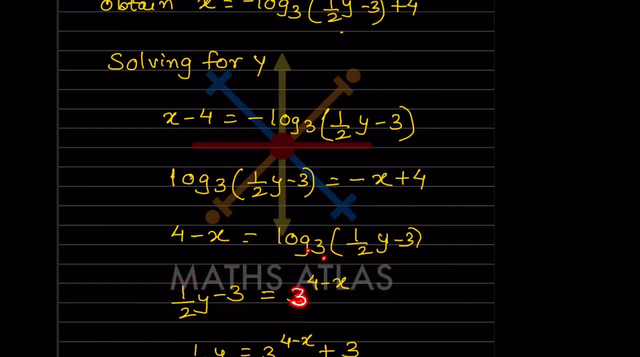 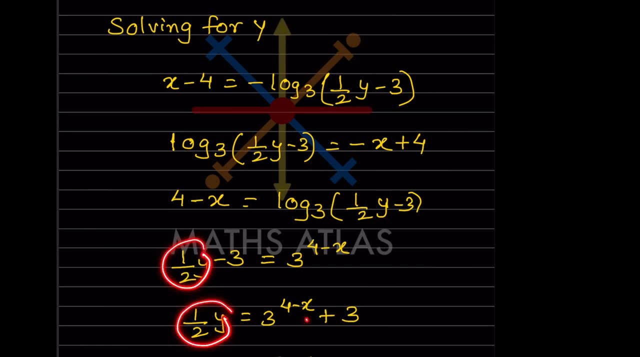 because this is log of 3. so you, you are going to follow the law. that will be 4 minus x. so now here, 1 by 2, this is y. so how will you write here? this will be same, minus 3 will go on the other side. that is going to be plus 3. so now this: what? 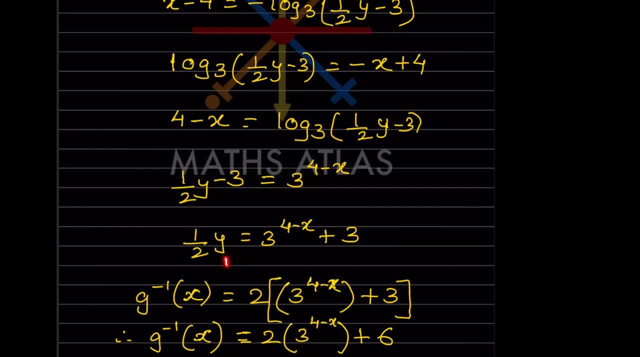 we can write here. we can also write one step over here. so y is 2, because this goes on the other side. so that is 1 by 2 is going to be 2 and this is going to be 3. raise to 4. you can write this step.